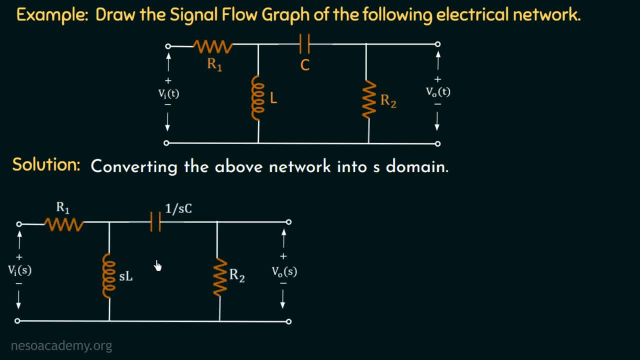 domain. then this network will look like this: See: the input voltage is VIS. the impedance of resistor is R1,. the impedance of this inductor is SL. the impedance of this capacitor is 1 over SC. the impedance of this resistor is 1 over SC. the impedance of this resistor is 1 over SC. 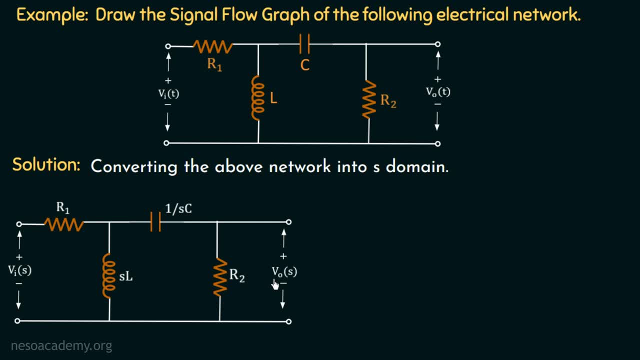 the impedance of this resistor is R2 and the output voltage which is measured across this resistor is Vout S. Now, if we observe this, output voltage is measured across this resistor R2 and hence the voltage at this node will be Vout of S. Similarly, the voltage at this node 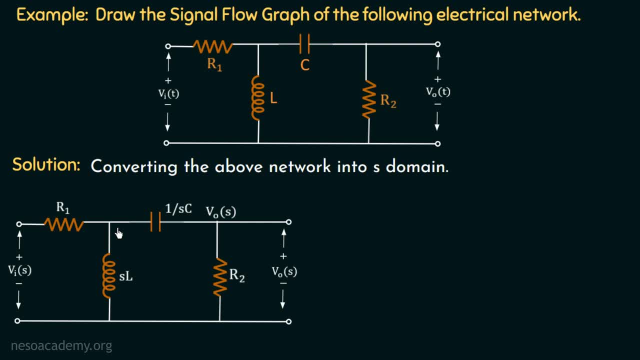 is the drop across this inductor. Let us assume that this node voltage is VL of S. Now we can see that this circuit has two different loops. So let us assume the current in this loop be I1S and the current in this loop equal to I2S. 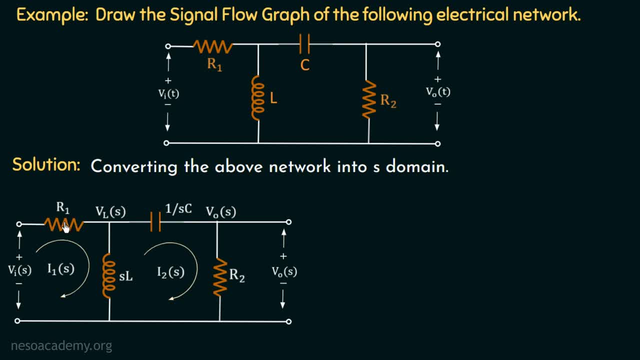 In this way, the current in this resistor will be I1S. the current in this inductor will be I1S minus I2S, and this is because I1S current is moving through this inductor in the downward direction and I2S current is moving through this inductor in the upward direction, And hence, 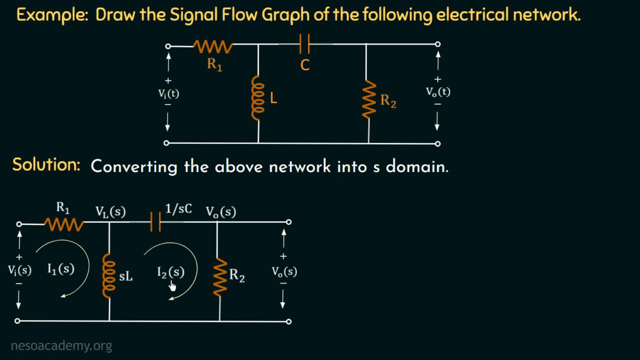 the net current downwards will be I1S. I hope you got this. Now we will move on to this capacitor. The current across this capacitor will be I2S and the same current is moving towards this resistor as the current through this open-circuited branch will be zero. So we can say that these two elements. 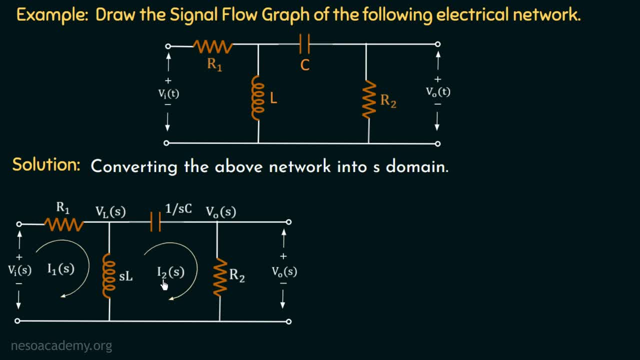 are in series and the current through these two elements is I2S. So in this way we are now aware of all the currents moving through the elements present in the circuit and the node voltages. We will now move on to the calculation of branch current equations and. 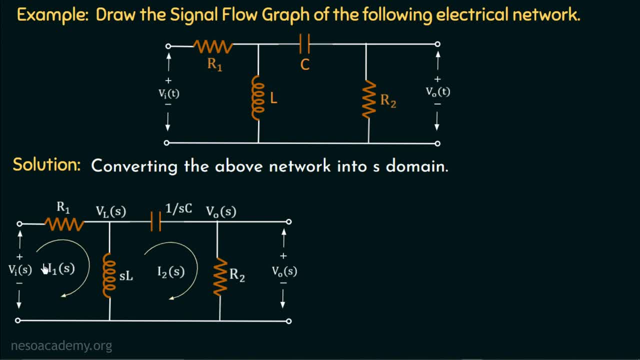 the node voltage equations. So let us start with the calculation of branch current I1S. We know that the current through this resistor is I1S and we can calculate this by applying Ohm's law in this resistor. The voltage at this terminal of resistor is Vi and the 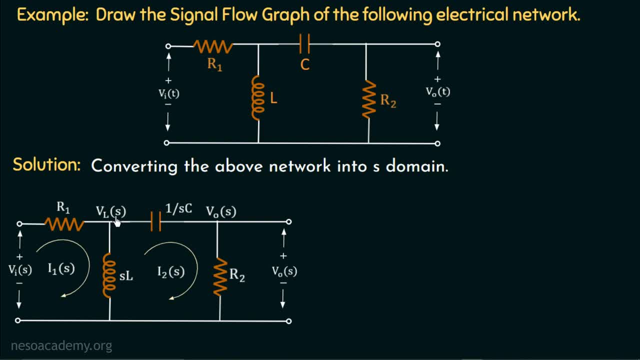 voltage at this node is VL. So if we apply Ohm's law to this resistor R1, we will have I1s equal to Vi of s minus Vl of s over R1, and if we split this we will have I1s equal to. 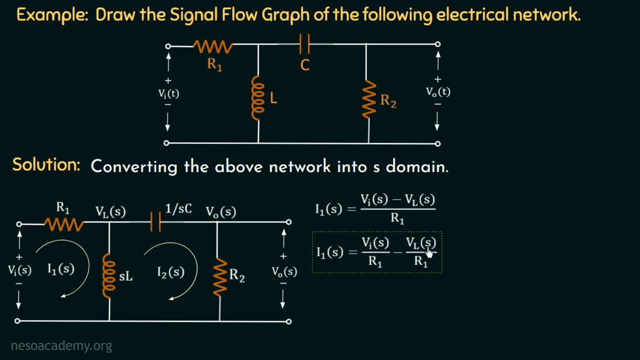 Vi of s over R1, minus Vl of s over R1, and this is the first branch current equation. We will now move on to the calculation of this node voltage equation and we know that this node voltage is the voltage drop across this inductor, and the voltage drop across this inductor will be the. 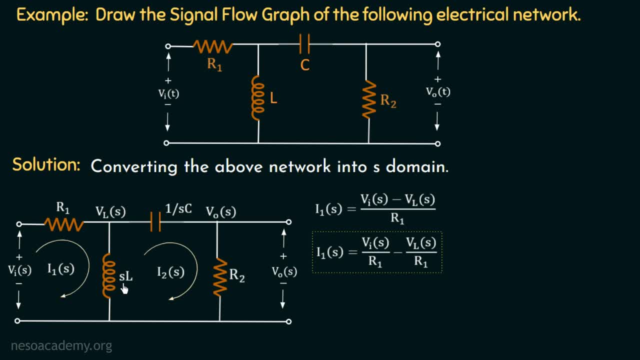 current passing through this inductor, multiplied with the impedance of this inductor. So we can write Vl of s, which is this node voltage, equal to I1s minus I2s, which is the current passing through this inductor, multiplied with sl, which is the impedance of this inductor. Let us check. 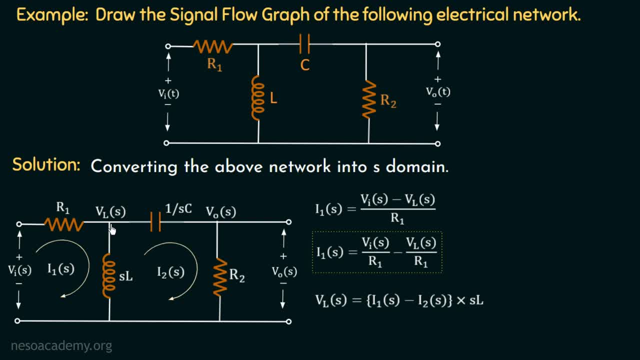 this out one more time: Vl of s is the node voltage and it is the voltage drop across this inductor. and we can calculate this by taking the product of current passing through this inductor multiplied with the impedance of this inductor, So the 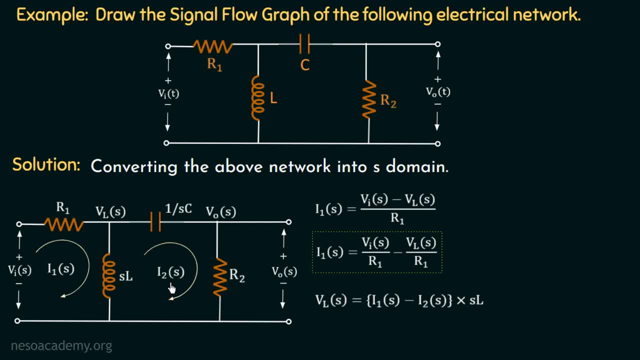 current passing through this inductor is I1s minus I2s- that we have already discussed- and the impedance of this inductor is Sl. Now, if we open this bracket, we will have the node voltage equation VL of s equal to I1s multiplied with Sl, minus of I2s multiplied with Sl, And in this way, 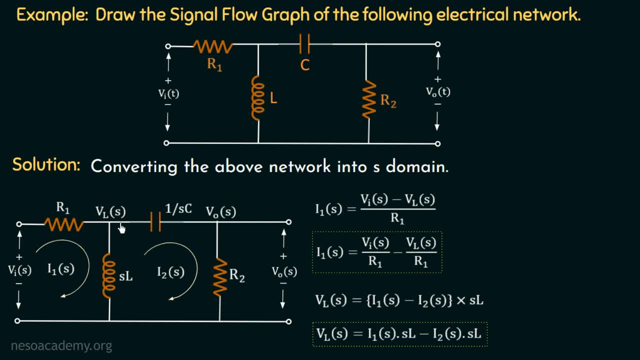 we are now done with the calculation of node voltage equation by calculating the value of VL of s. We will now move on to the calculation of second branch current equation by calculating the value of I2s, And we can calculate this by applying the Ohm's law in this capacitor. 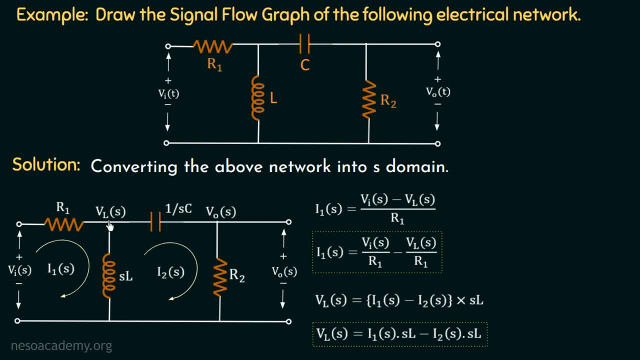 We know that the voltage at this terminal of capacitor is VL of s and the voltage at this terminal is V out of s. The current passing through this capacitor is I2s and the voltage at this terminal is V out of s And the impedance of this capacitor is 1 over Sc. So if we apply, 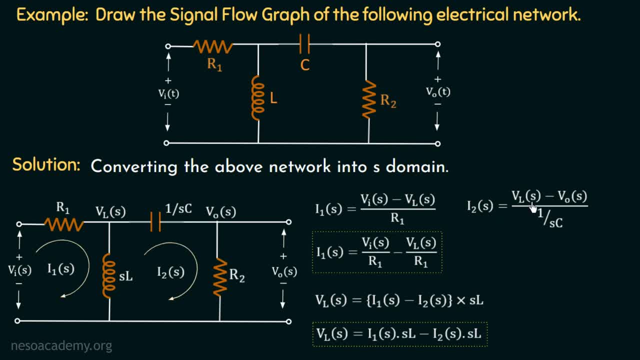 the Ohm's law expression to this capacitor, we will have I2s equal to VL of s minus V0 of s, which is the difference of voltages over the impedance of capacitor, which is 1 over Sc. This is the Ohm's law expression for this capacitor in Laplace domain. Now, if we solve this this term, 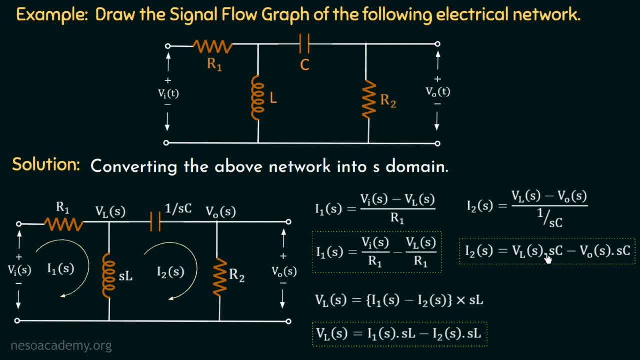 will come to the numerator and we will have VL of s multiplied with Sc, minus V0 of s multiplied with Sc, And in this way we are now done with the calculation of second branch current equation. We will now move on to the last equation. 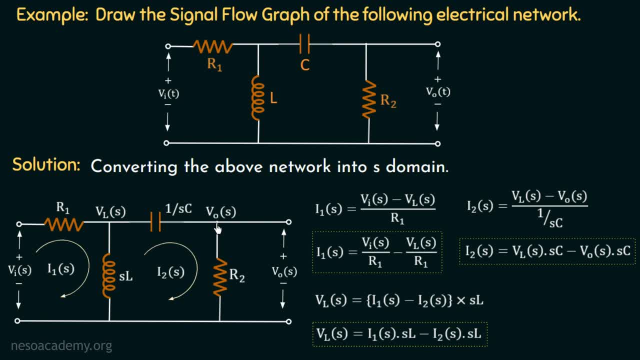 which is the node voltage equation at this node. For that sake, we have to calculate the value of V out of s. We know that V out of s is the voltage drop across this resistor. And if we want to calculate the voltage drop across this resistor, we have to take the 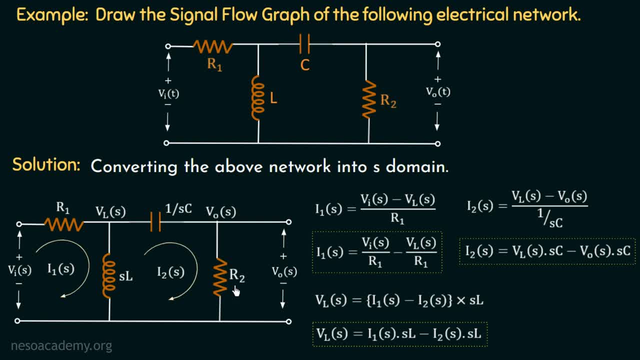 product of current passing through this resistor and the impedance of this resistor. So we will have V out of s equal to I2s multiplied with R2.. I2s is the current passing through this resistor, R2 and R2 is the impedance of this resistor. And this is our last node voltage equation. And in 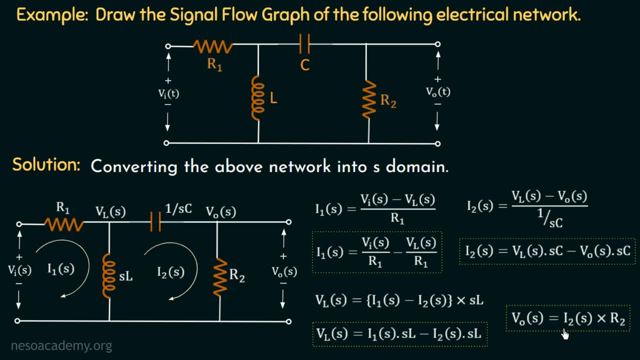 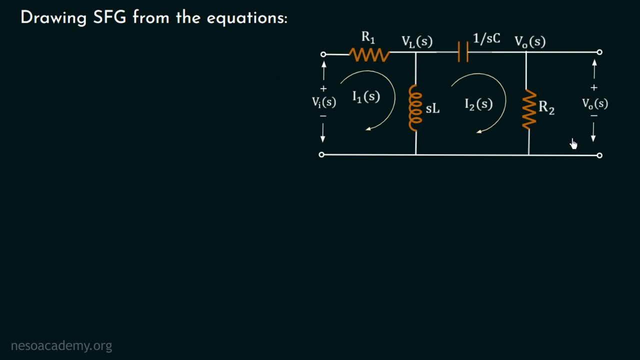 this way we have calculated all the branch current equations and the node voltage equations. We will now use these linear equations in order to draw the the signal flow graph. Let us now move on to the drawing of signal flow graph from the equations that we calculated. This is the electrical network given in the example and these are the equations. 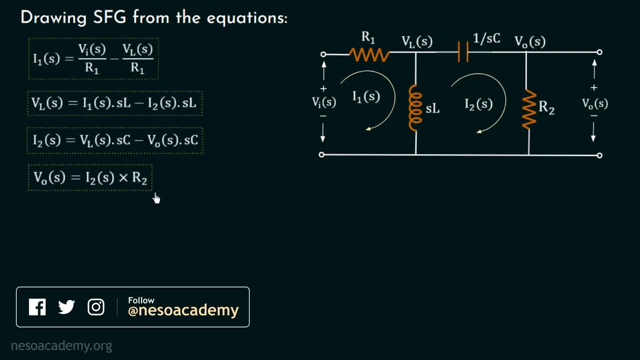 that we have calculated in the previous section. Now we will use these equations in order to draw the signal flow graph of this electrical network. So the first step is to calculate the number of nodes in the signal flow graph. So what will be the number of nodes in the signal flow graph? 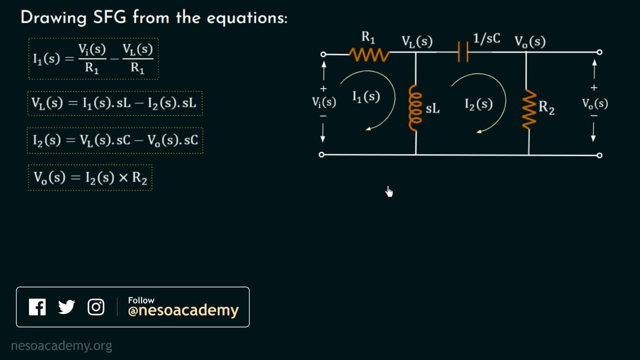 Yes, the number of nodes is equal to the number of variables present in the electrical network. If we count the number of variables, we can see the first variable is vi of s, the second variable is i1 of s, the third variable is vl of s, the fourth variable is i2 of s and the fifth variable 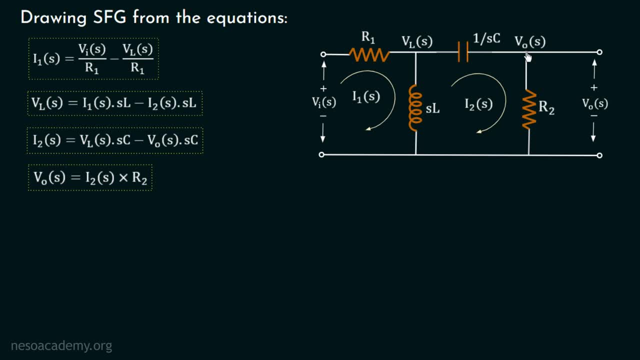 is vout of s. So in this way we have five variables present in this electrical network and that's why we have the number of nodes present in the electrical network. We will have five nodes present in the signal flow graph. The first variable is vi of s. the second 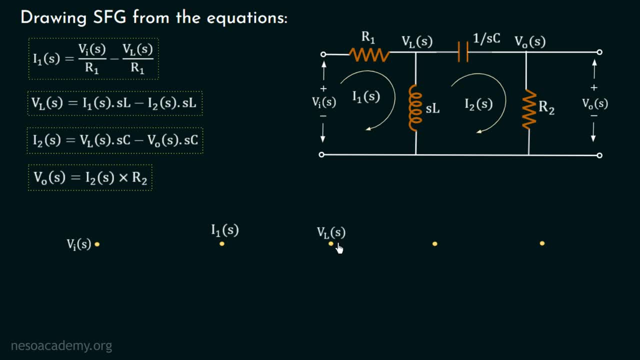 variable is i1 of s, the third one is vl of s and similarly, the fourth one is i2 of s and the last one is vout of s. We can observe one important point here in the pattern of nodes: The first one is a voltage variable, the second one is a current variable. the third one is a voltage variable. 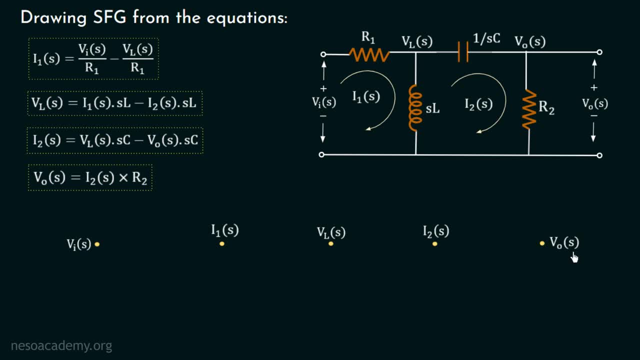 fourth one is a current variable and the last one is a voltage variable. We can see that the voltages and current variables are present in an alternate fashion. So this is an important observation here. We will use this in the later section of this lecture. So we are done with the 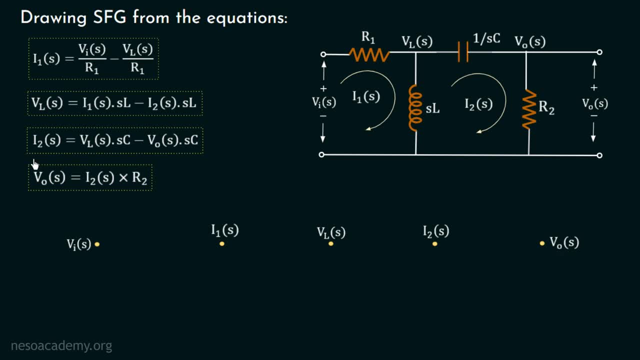 first step, which is the plotting of nodes. We will now use these equations in order to relate these nodes. So if we observe this first equation, i1 is equal to vi of s over r1, minus vl of s over r1.. We can see that this equation relates this node i1s with this node vis and this node. 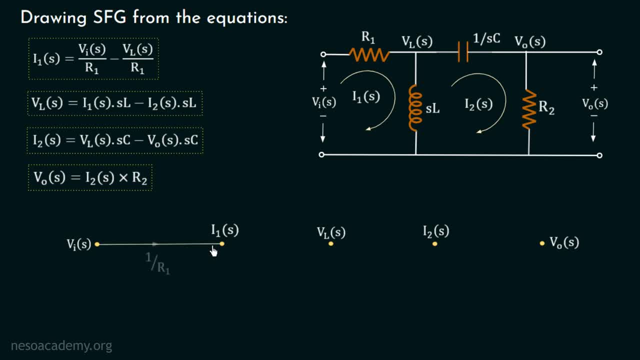 vl of s, And we can see that i1 of s is vi of s multiplied with 1 over r1, minus of vl of s multiplied with 1 over r1.. And in this way we have one forward path and one negative feedback. 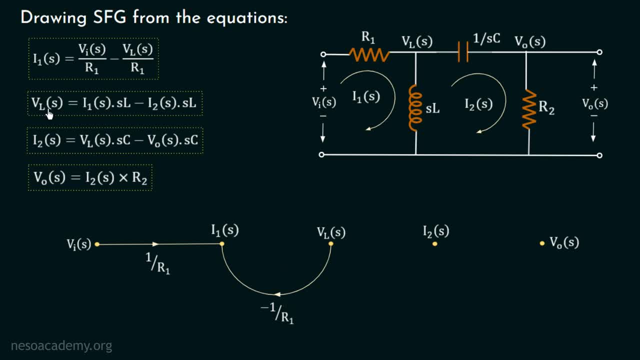 path. Let us now move on to the second equation, which is vl of s equal to i1s multiplied with sl, minus i2s multiplied with sl. We can see that this equation relates this node, vl of s, with these two nodes, i1s and i2s. We can see that vl of s is i1s multiplied with sl. 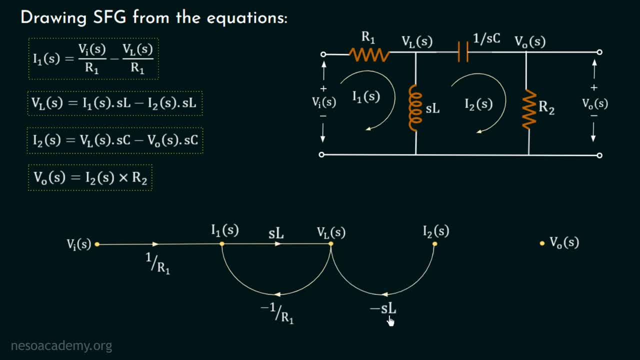 minus i2s multiplied with sl. In this way again, we have one forward path and one negative feedback path by using this second equation. Let us now move on to the third equation, which is i2s equal to vls multiplied with sc, minus vout s multiplied with sc. We can see that. 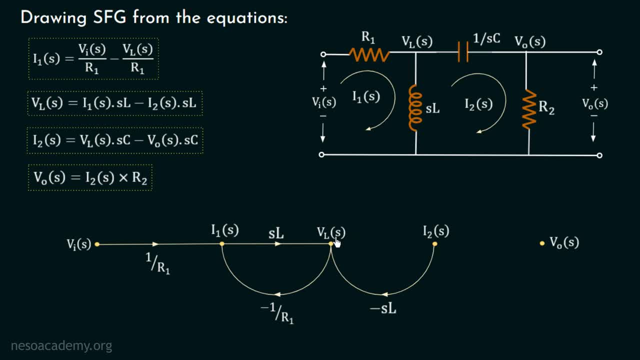 this equation relates this node, i2s, with these two nodes, vl of s and vout of s, And we have i2s equal to vls multiplied with sc, minus vout of s multiplied with sc. And in this way, again, we have one forward path and one negative feedback path. 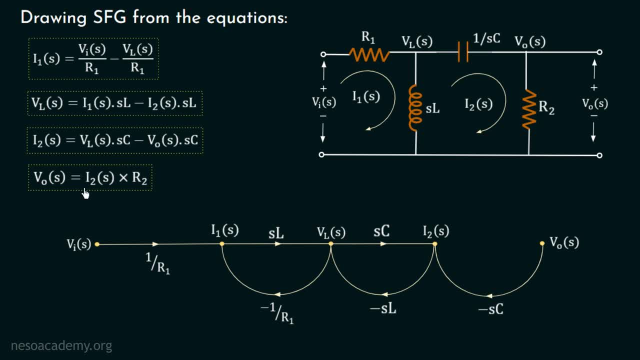 by using this second equation, Let us now move on to the third equation, which is i2s equal to vls. using this third equation, Let us now move on to the fourth equation, which is vout s equal to i2s multiplied with r2.. We can see that this equation relates this output node, vout s, with this node. 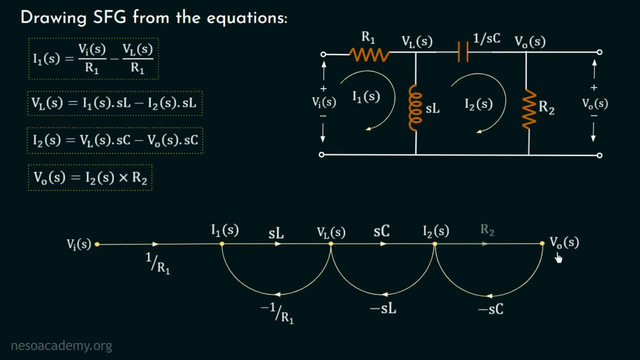 i2s, And we can see that vout s is equal to i2s multiplied with r2.. And in this way we have only one forward path by using this fourth equation, And this is the complete signal flow graph of this electrical network. 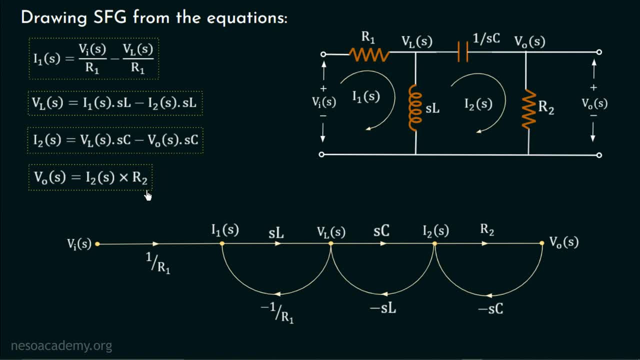 And we have drawn this by the use of these four linear equations. Let me tell you one important observation here: When we were using this first equation, we had one forward path and one negative feedback path. Similarly, when we were using second equation, we had one. 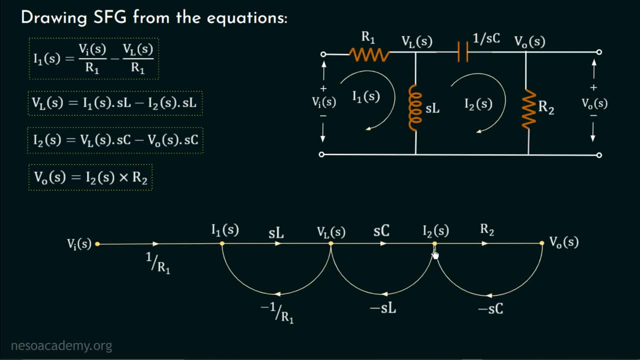 forward path and one negative feedback path. In the same way, when we were using the third equation, we had one forward path and one negative feedback path, But when we use this fourth equation, we had only one forward path and no negative feedback path. So this is an important 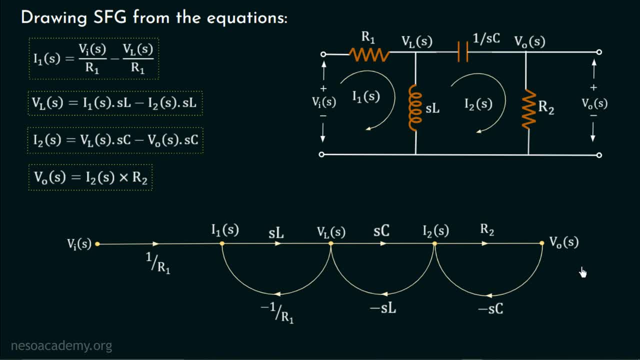 observation. We will use this in the later section of this lecture. So till now we have discussed that how we can calculate the branch current equations and the node voltage equations for a given electrical network and how we can use these linear equations in order to draw the signal flow. 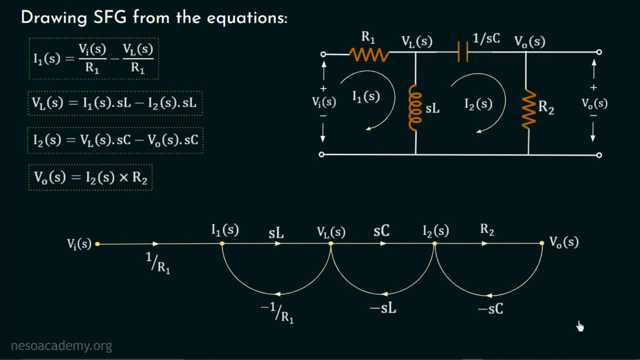 graph of any electrical network. We will now discuss a shortcut method by which we can draw the signal flow graph directly from the electrical network without using these linear equations. So we do not have to calculate the branch current equations and the node voltage equations if we use the shortcut method. Are you excited for this? So let's dive into it. Moving on. 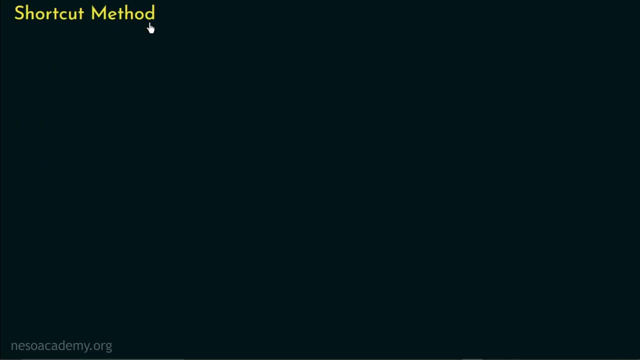 to the shortcut method by which we can draw the signal flow graph directly from the electrical network without using the linear equations. In this way, we do not have to calculate the branch current equations and the node voltage equations. we can directly draw the signal flow graph. 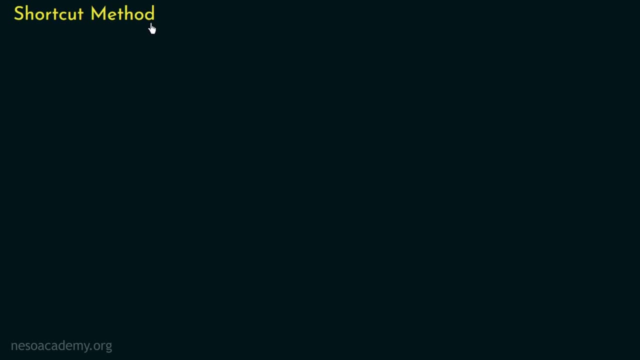 So, in order to use this method, we have to remember some important points. The first point is: all the network elements represent one forward path and one negative feedback, except the last element, And from the last element we refer the element from where we take the output. 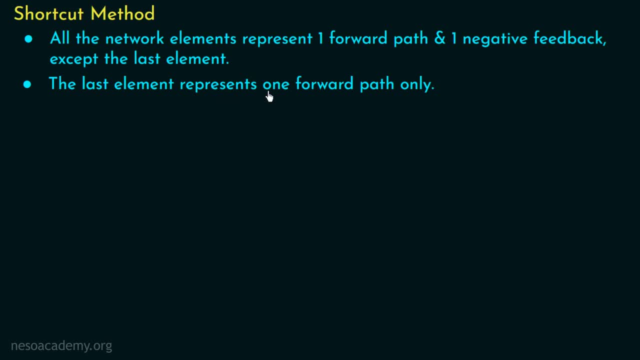 Moving on to the next point, the last element represents one forward path only, and it does not represent any negative feedback path. Moreover, in signal flow graph that we will draw directly from the electrical network, all the branch gains represent either the admittance or impedance in alternate form. 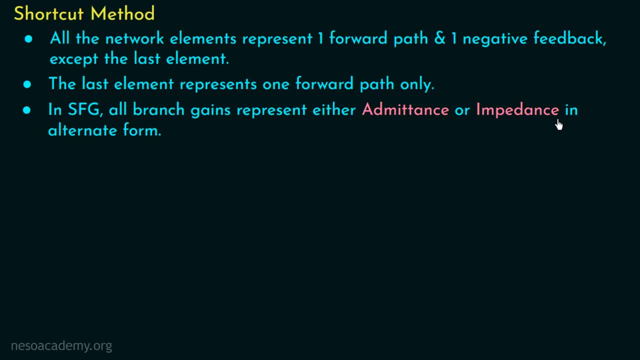 We already know the impedance right. It is the measure of overall opposition of an element to the current passing through it. So the admittance is just opposite to that of impedance. Admittance is the measure of how easily a device or a circuit can pass through it. 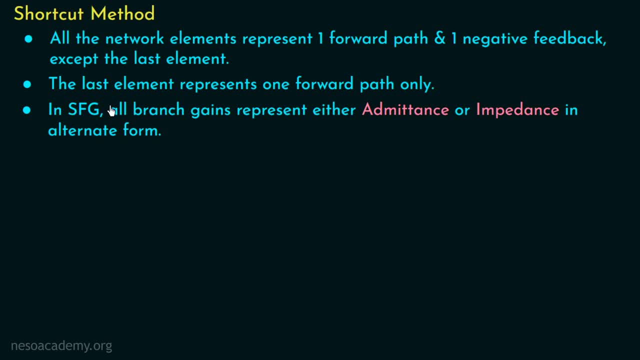 It allows a current to flow through it. So in the signal flow graph, all the branch gains represent either admittance or impedance in alternate form. Let us now consider the same example that we have discussed in this lecture, in which we have four elements. 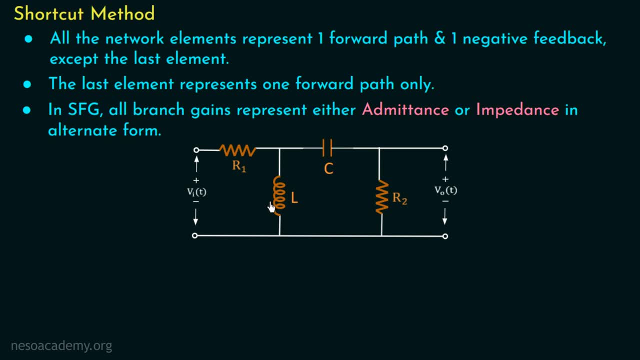 The first element is the resistor R1.. The second element is the inductor L, The third element is the capacitor C And the fourth element is the resistor R2.. The input voltage is ViT and the output voltage is VoutT, which is measured across this resistor. 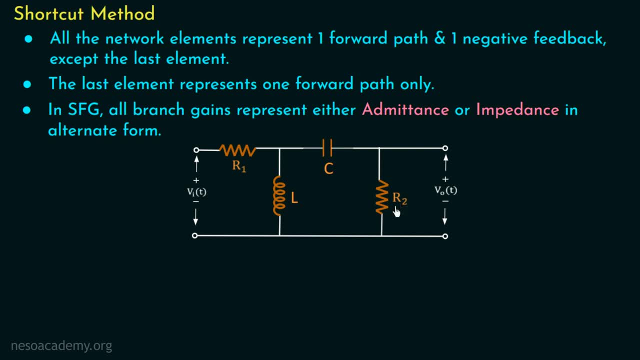 R2.. Now, according to the shortcut method, all the elements represent one forward path and one negative feedback, except the last element, And which is the last element of this network. Yes, this resistor R2 is the last element of this network, because we are taking the 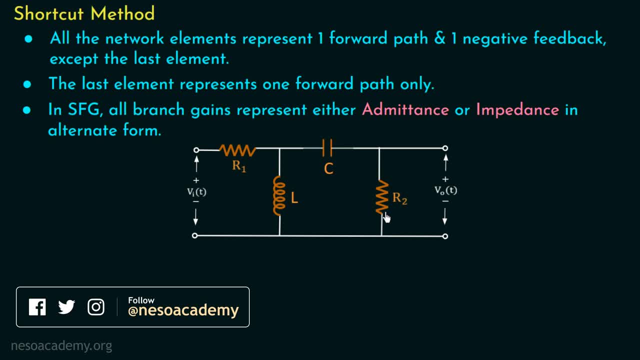 output across this resistor. So we can say that These three elements represent one forward path and one negative feedback. These three network elements will represent one forward path and one negative feedback in their equivalent signal flow graph representation, But this element, which is the last element, will represent only one forward path. 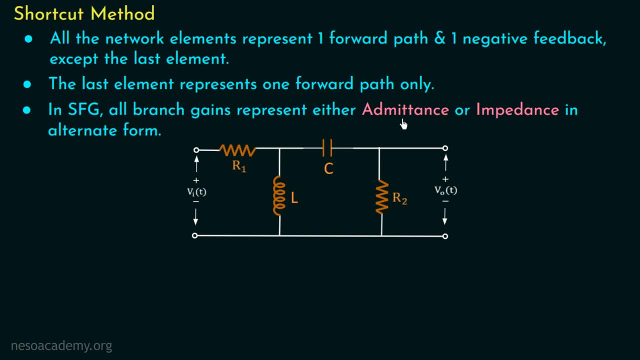 Moreover, all the branch gains represent either admittance or impedance in alternate form. So this resistor will represent its admittance in the signal flow graph. representation: This inductor will represent its impedance. Now, this capacitor will represent its admittance. And, lastly, this resistor will represent its impedance in its equivalent signal flow graph. 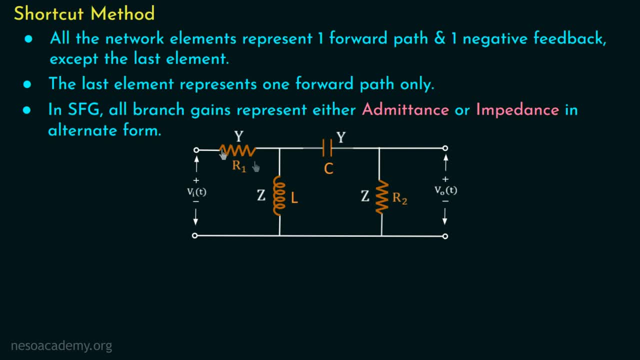 representation. We can remember this with this trick: All the elements which are present in horizontal position in the electrical network will represent their admittances in their equivalent SFG representation, And all the elements which are connected in a vertical position will represent their impedances. 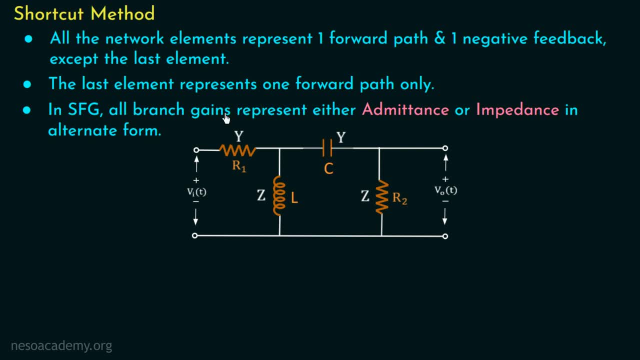 So I hope you got all the information in this video. Thanks for watching. If you liked this video, don't forget to like, share and subscribe to my channel, And if you want to see more such videos, click on the bell icon. 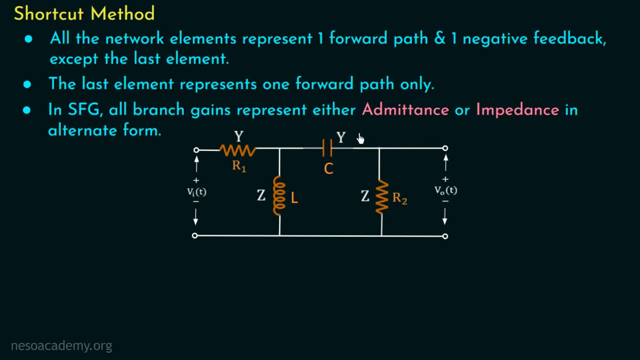 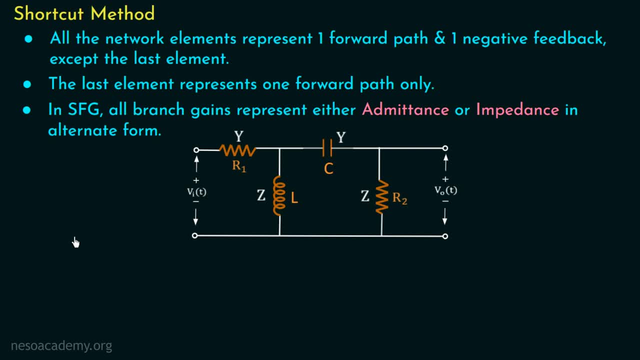 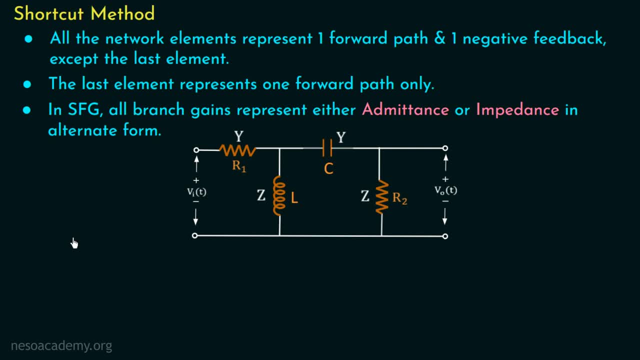 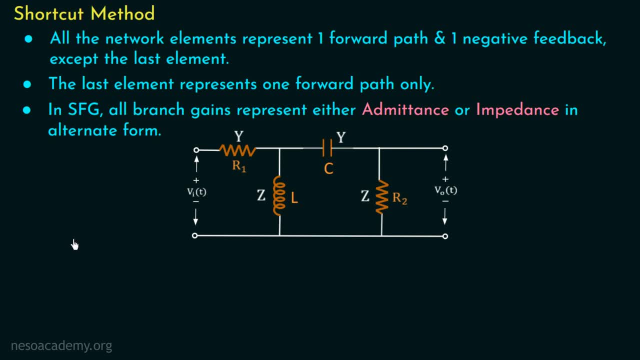 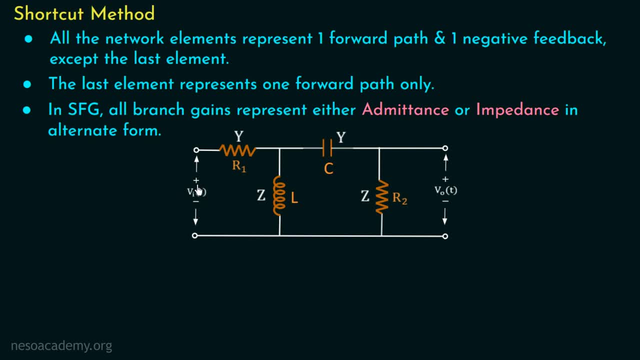 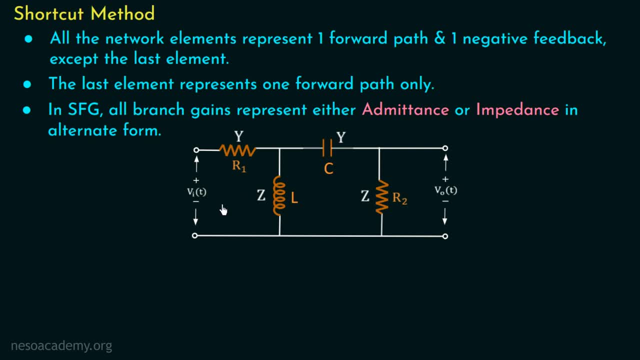 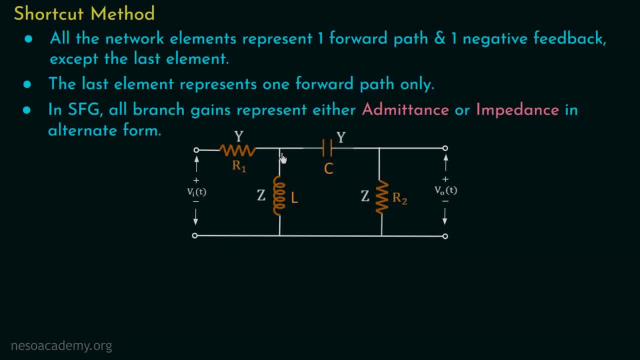 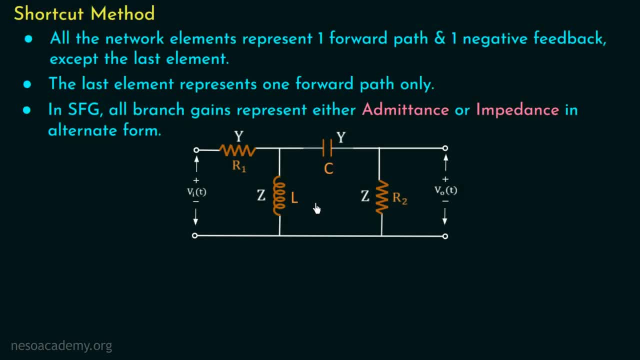 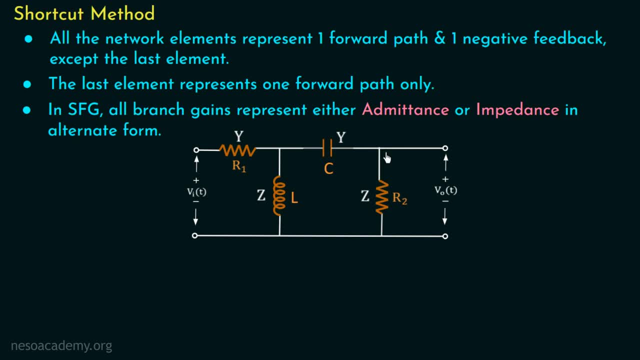 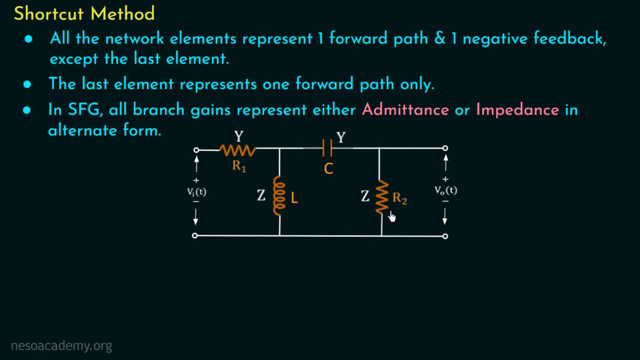 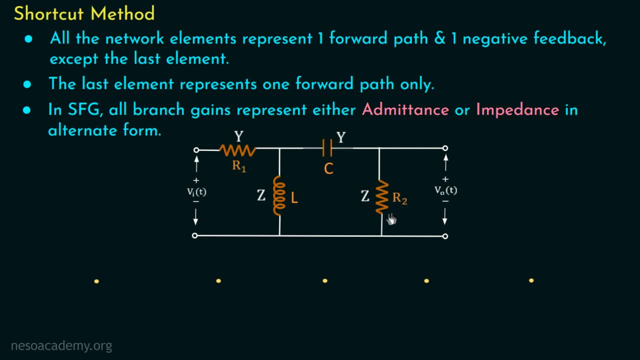 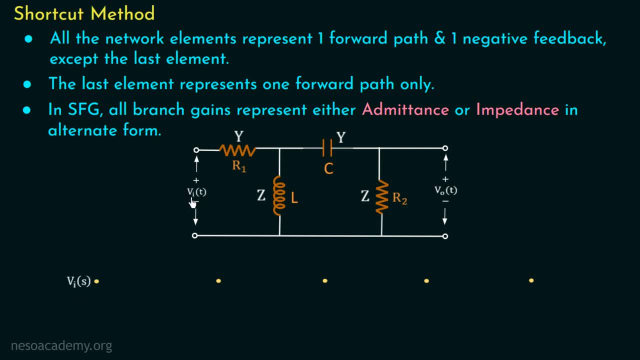 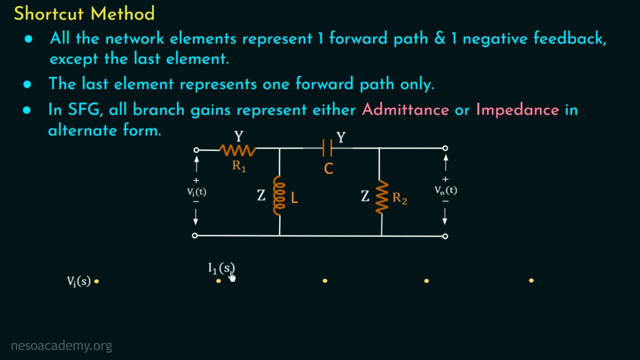 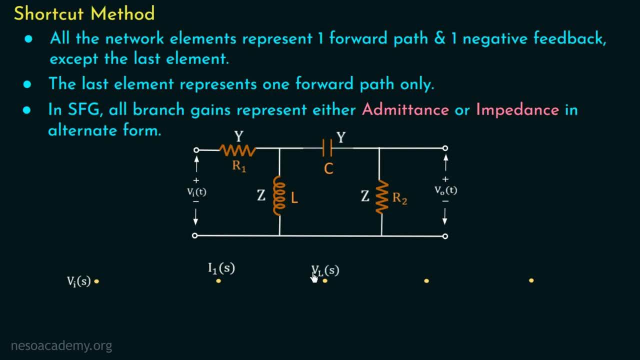 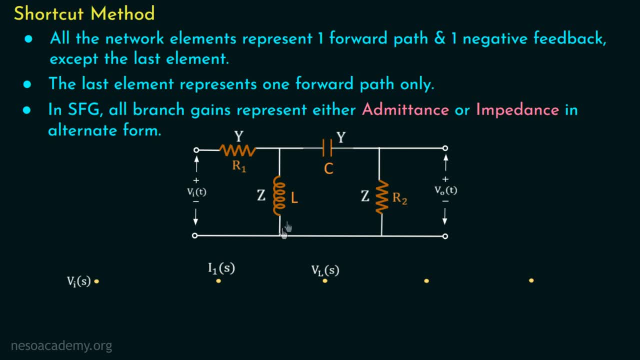 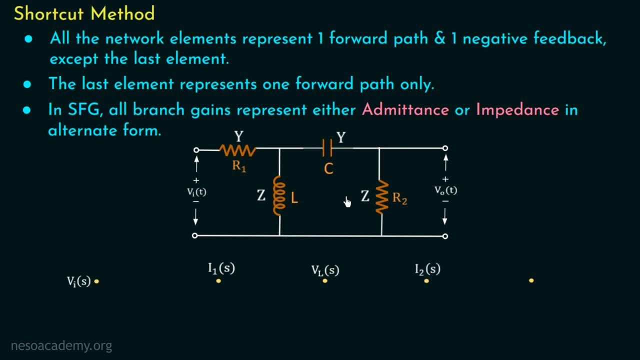 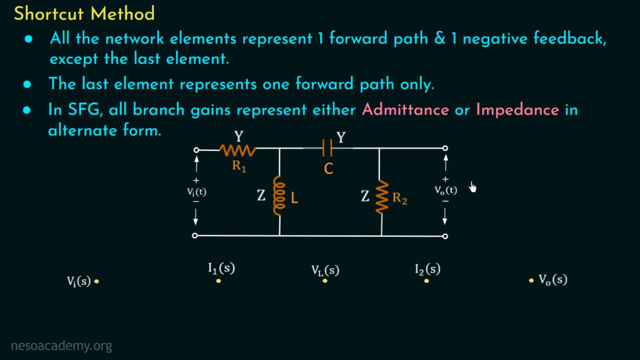 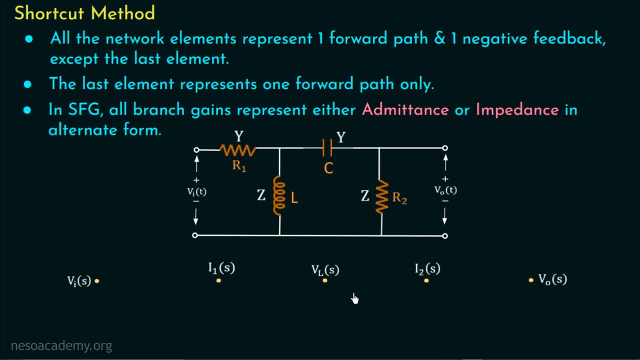 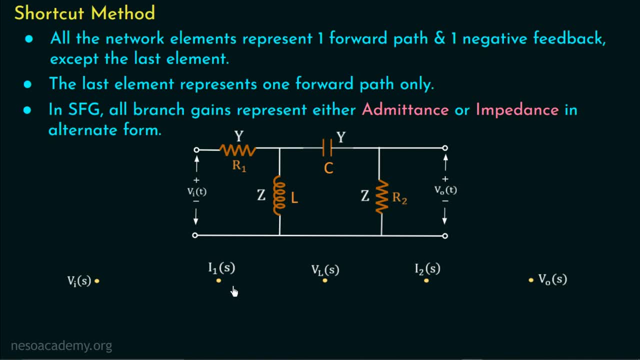 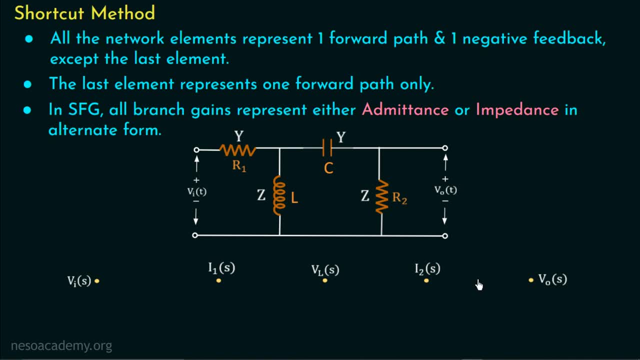 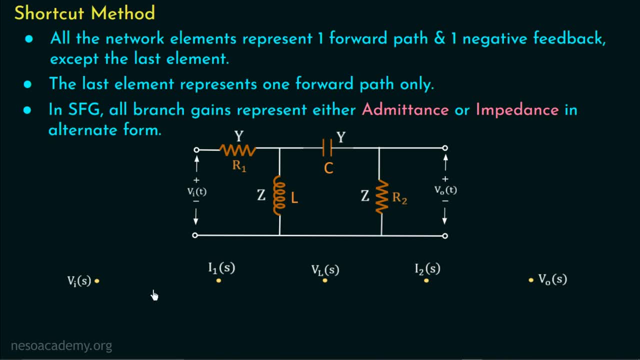 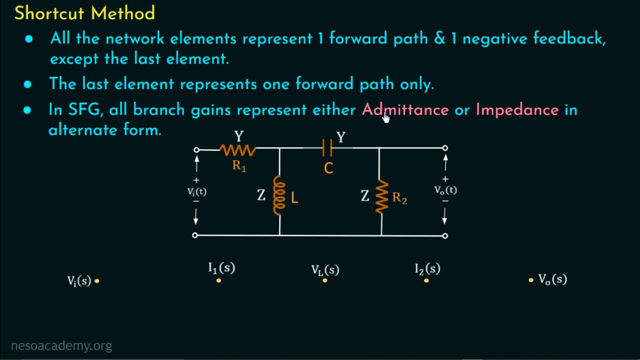 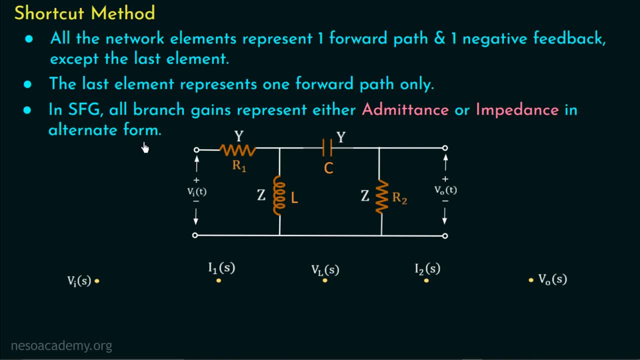 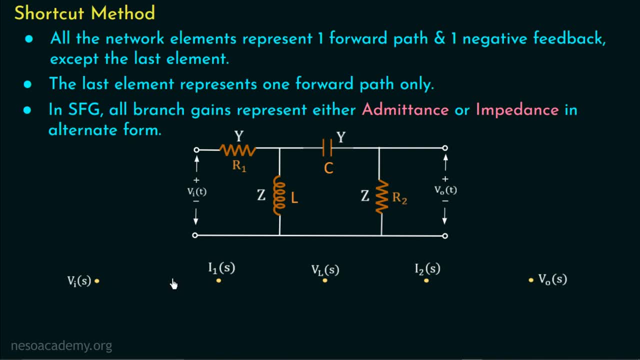 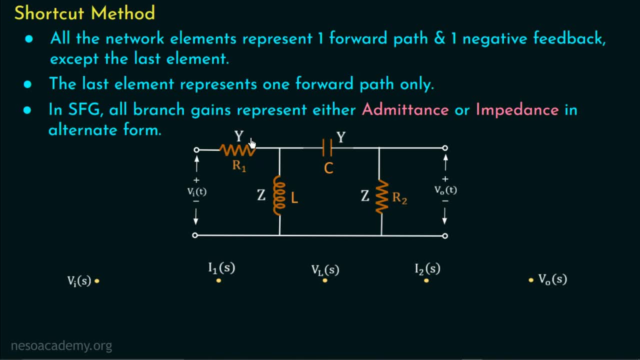 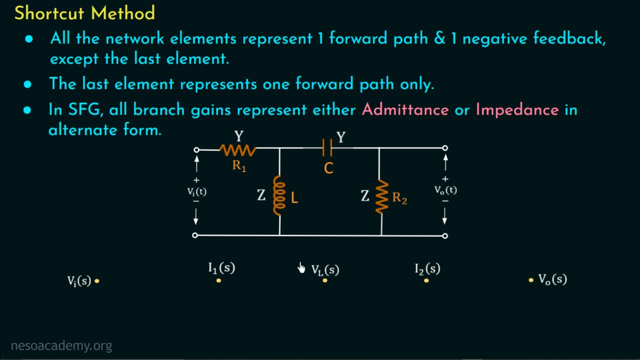 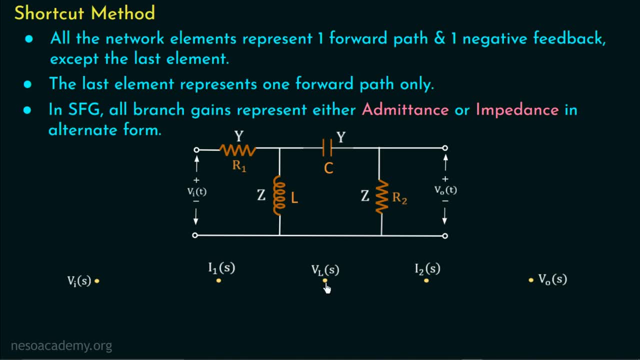 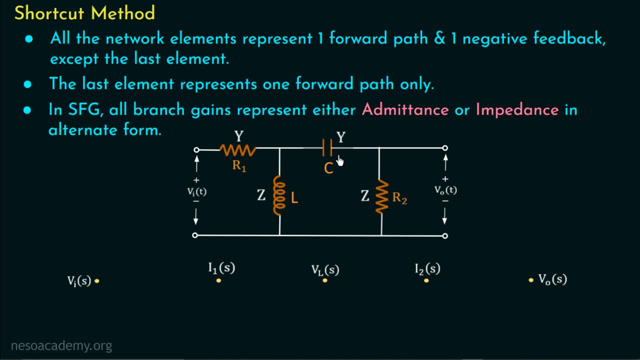 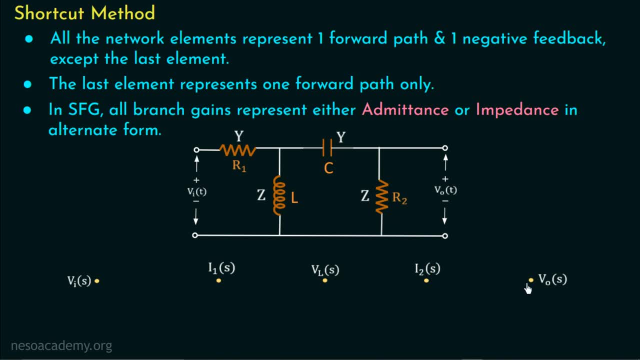 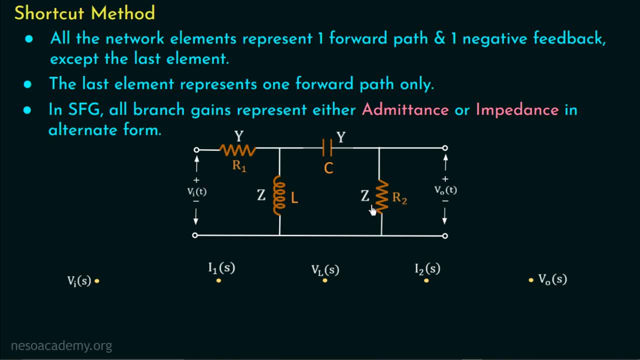 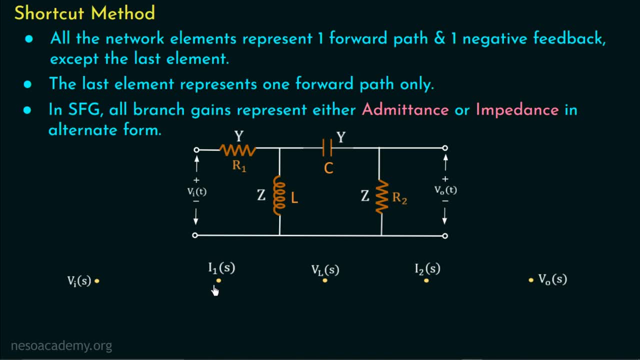 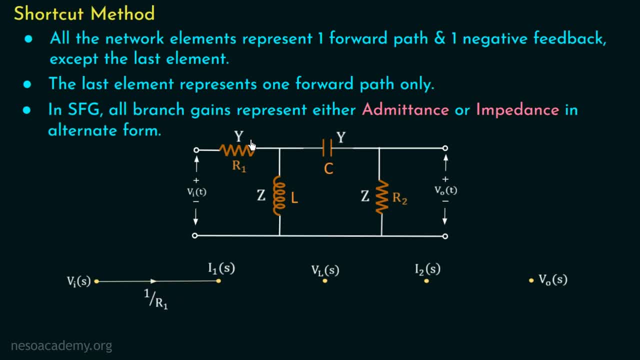 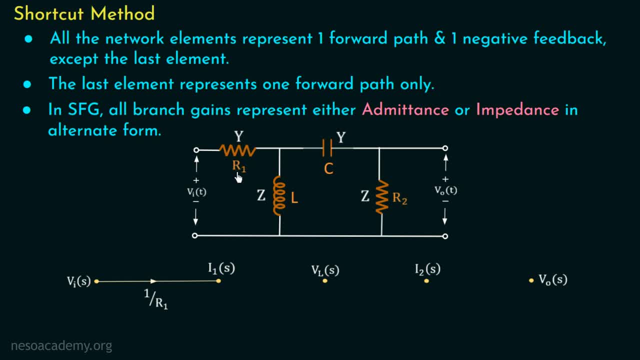 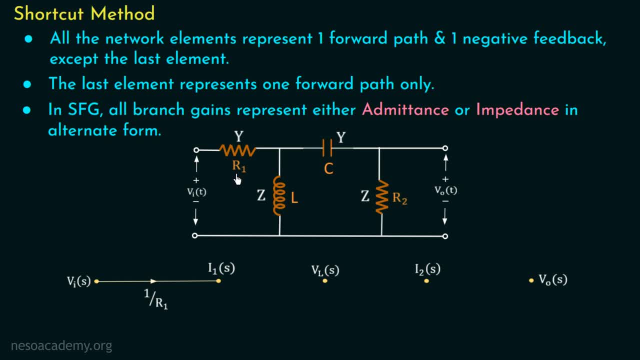 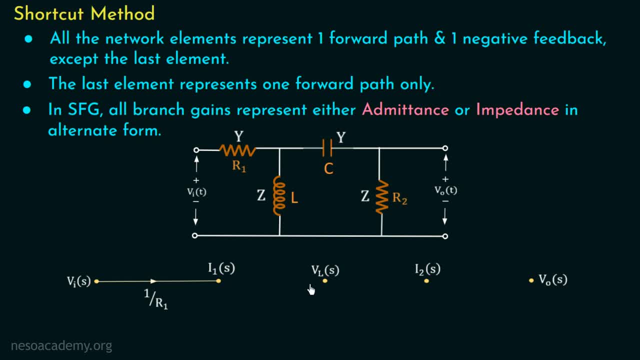 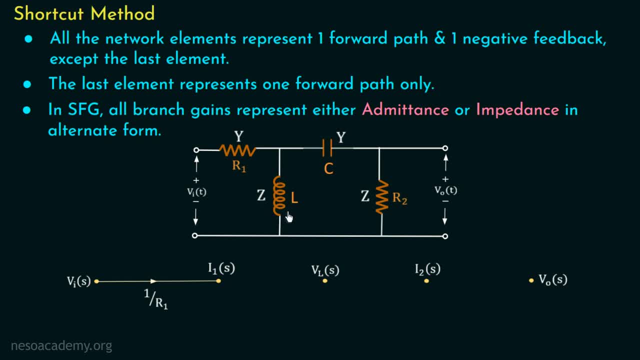 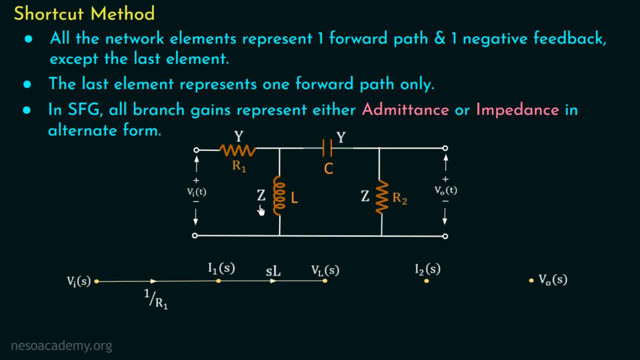 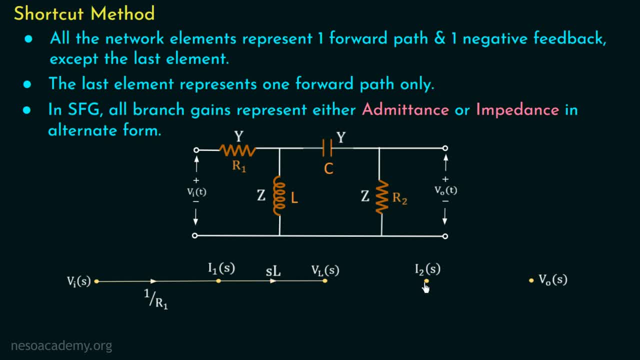 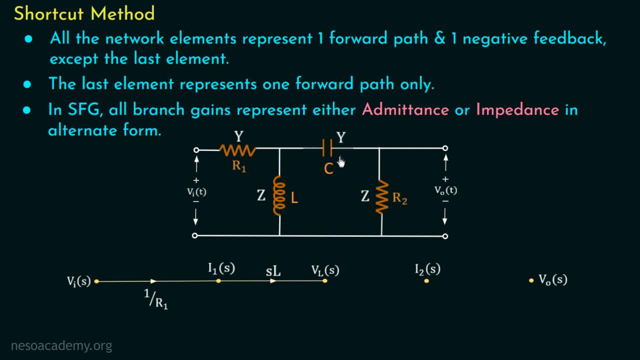 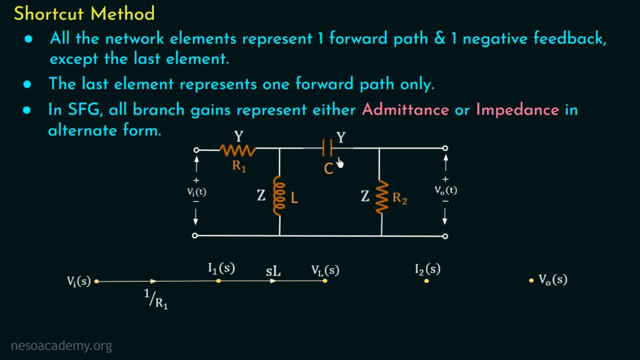 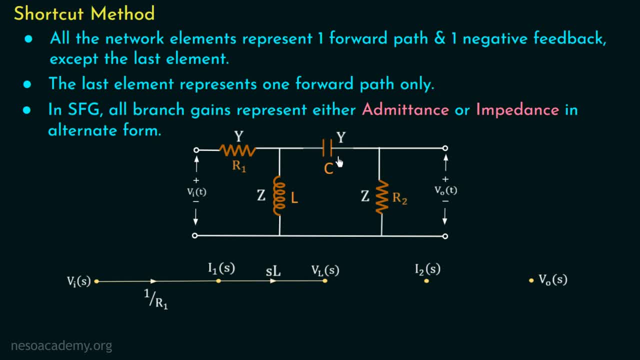 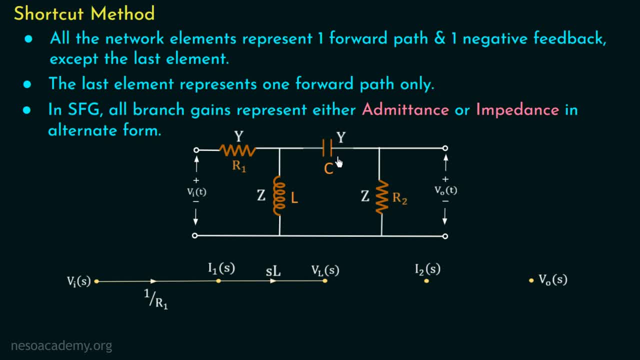 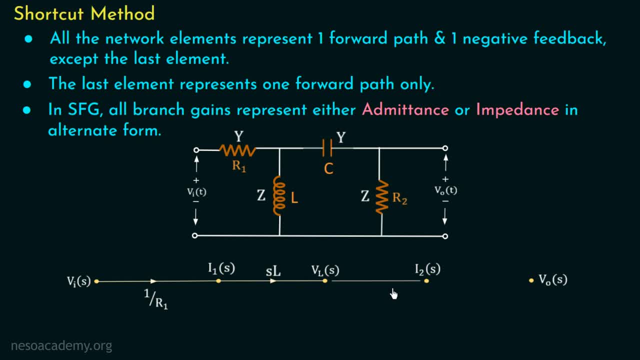 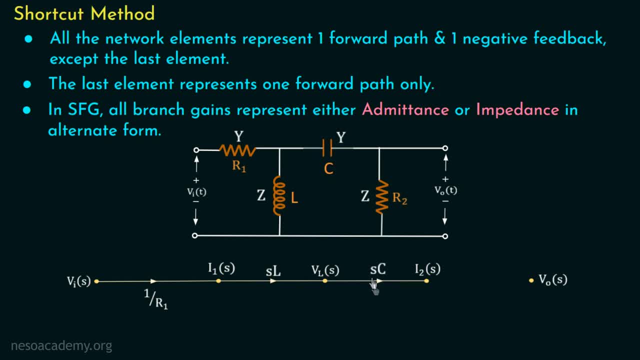 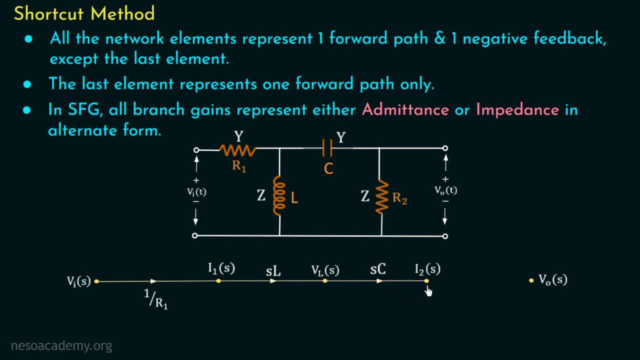 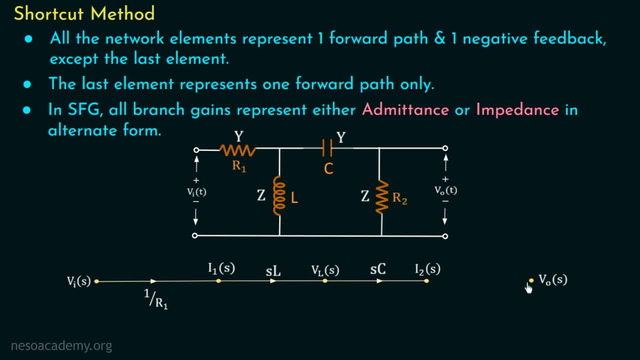 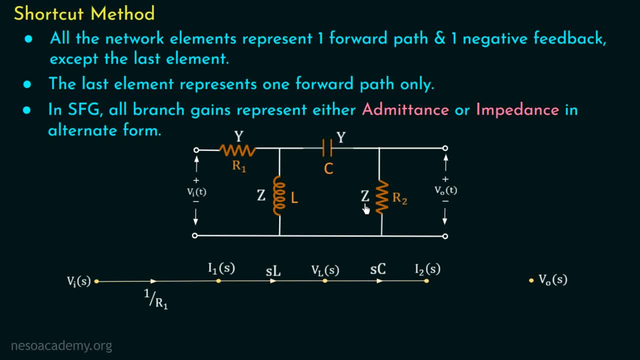 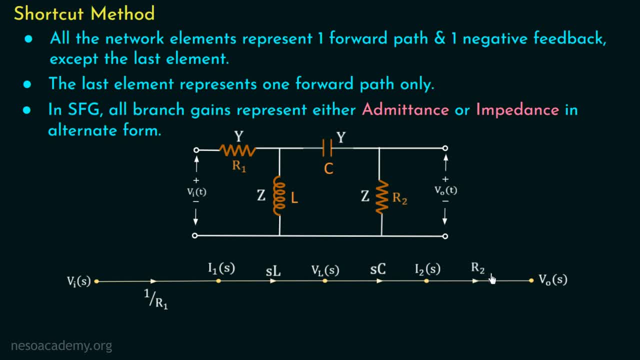 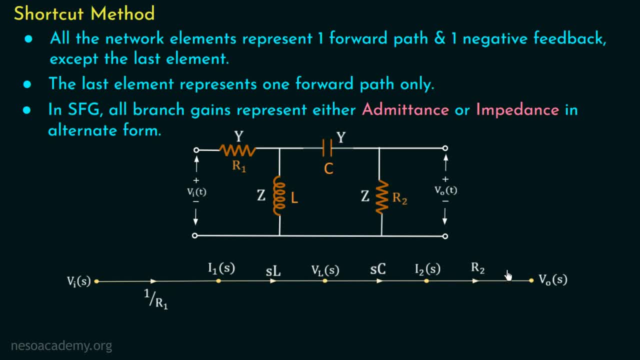 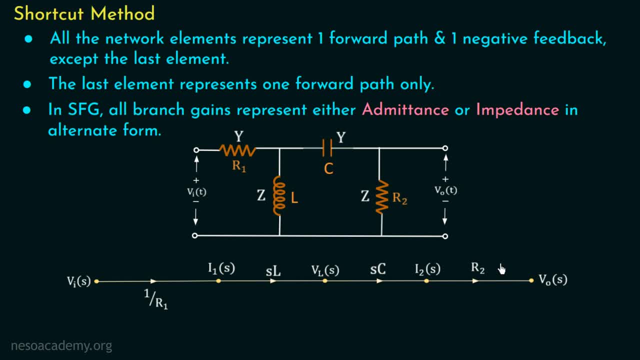 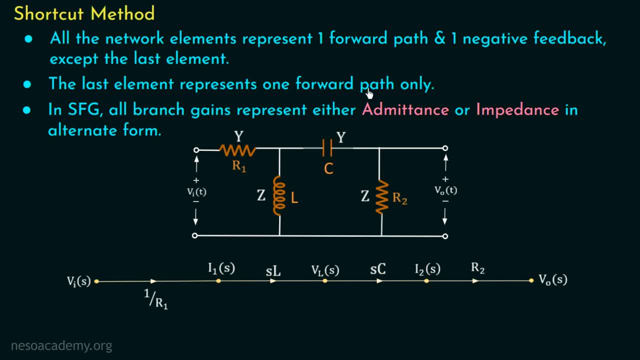 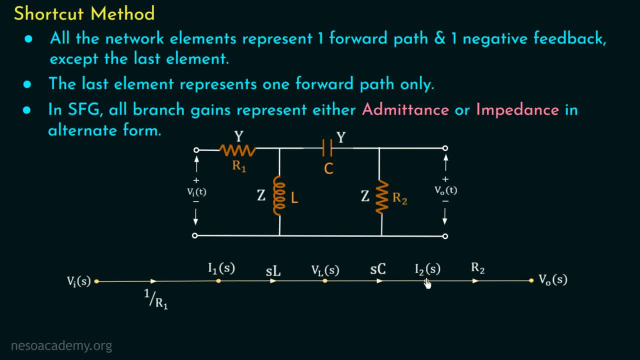 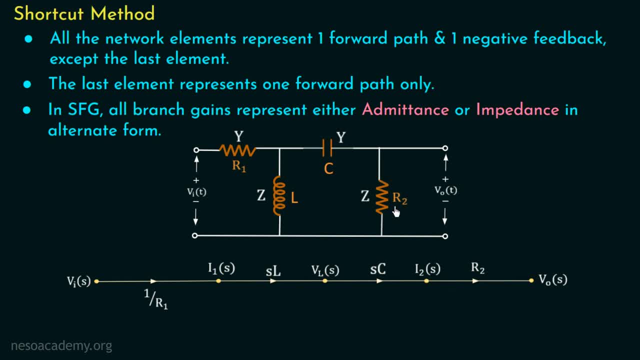 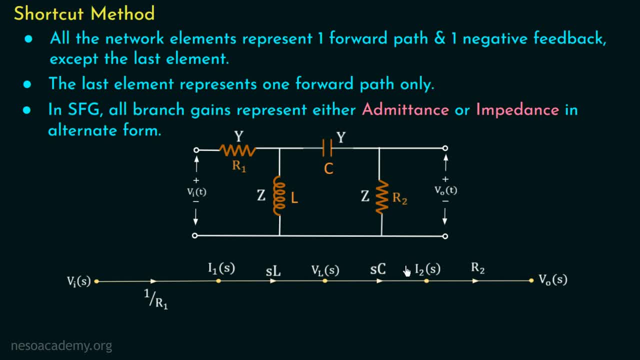 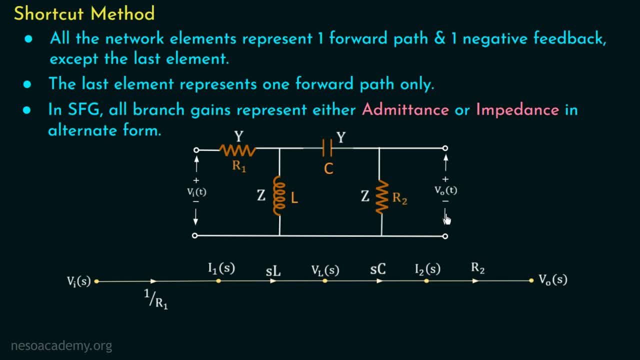 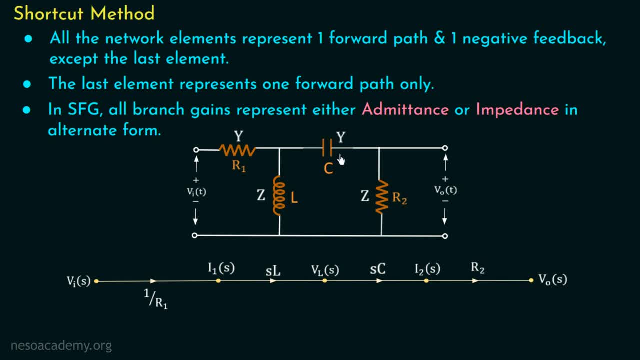 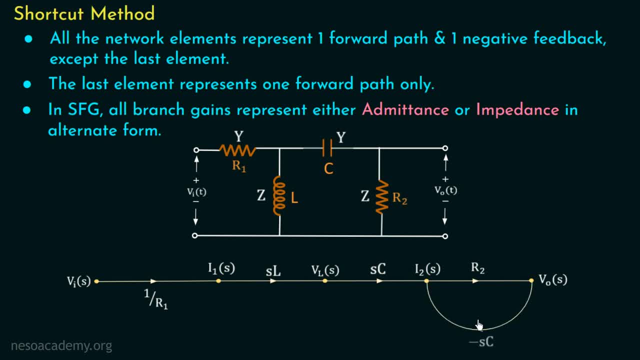 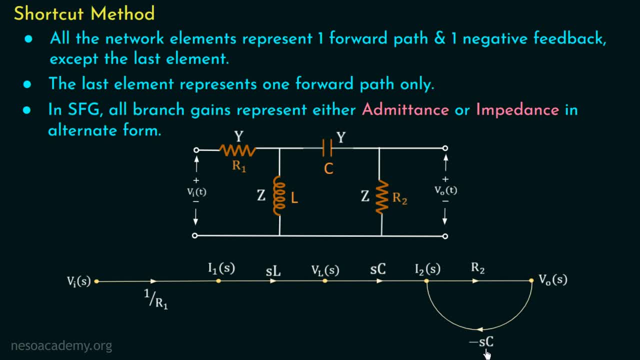 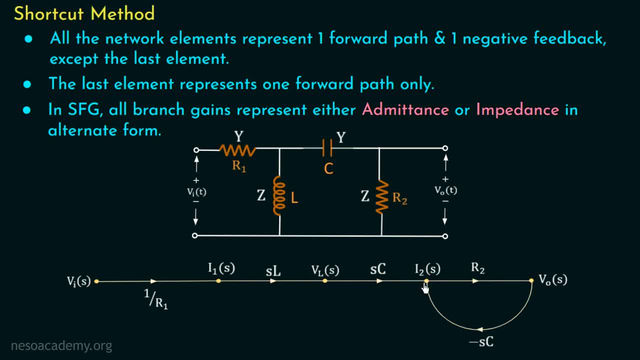 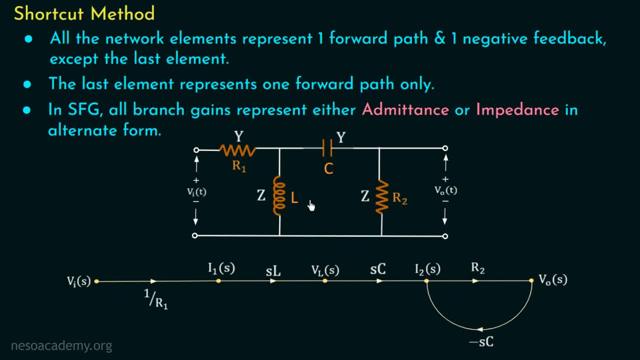 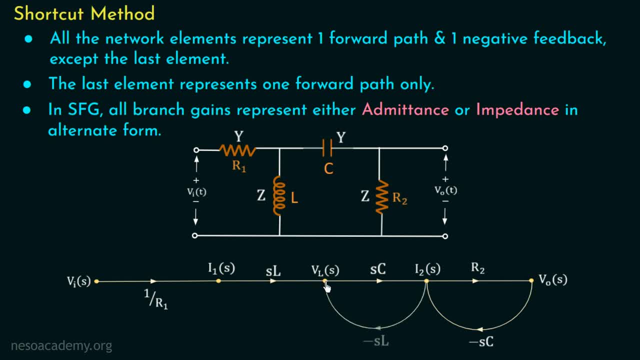 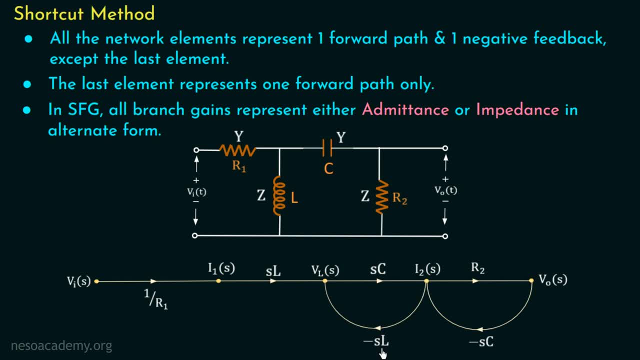 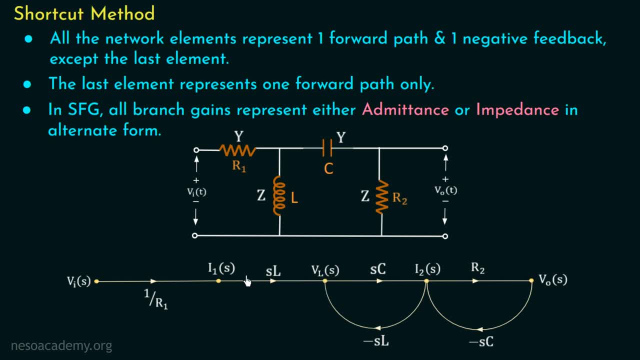 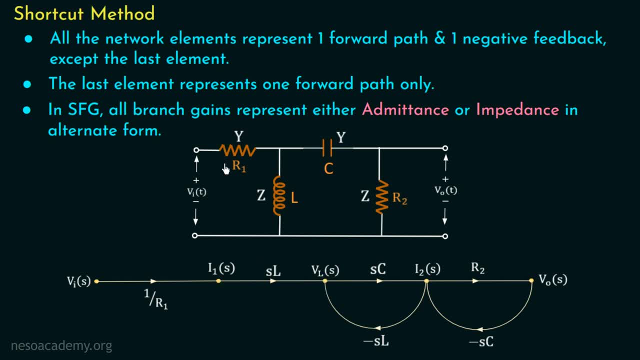 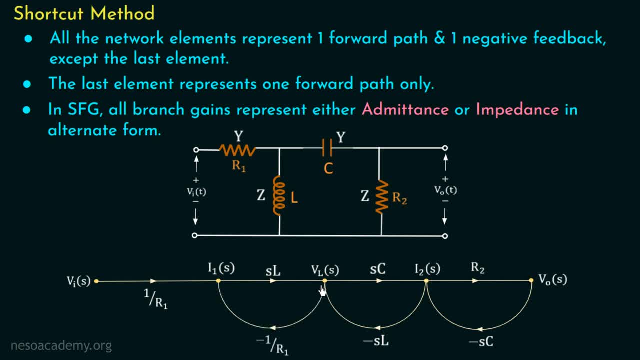 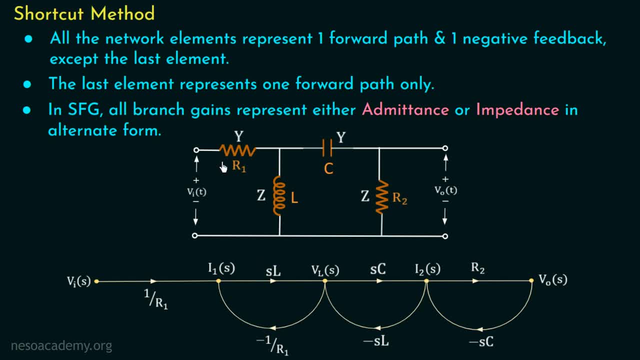 And if you want to see more such videos, click on the bell icon. And if you want to see more such videos, click on the bell icon is the admittance of this element. I hope you got this. let me repeat this one more time. 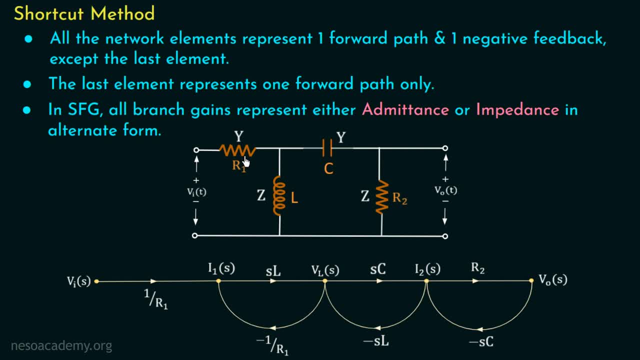 If we draw the signal flow graph for this electrical network, firstly we have to count the number of nodes, and we know that the number of nodes is equal to the number of variables. In this electrical network, the number of variables is equal to 5, and hence the number. 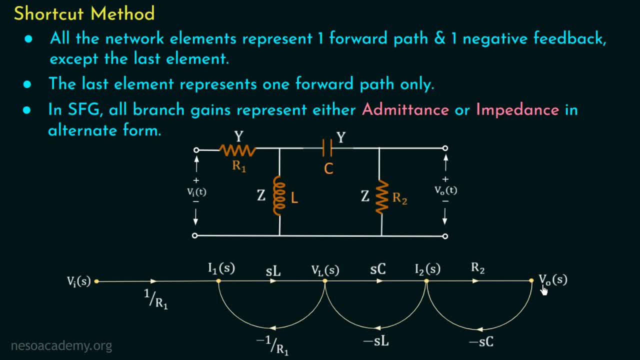 of nodes is also equal to 5.. Now, firstly, we have to draw the forward path and we know all the branch gains represent either admittance or impedance. So, firstly, whenever we are connecting these two nodes, the branch gain will be the admittance. 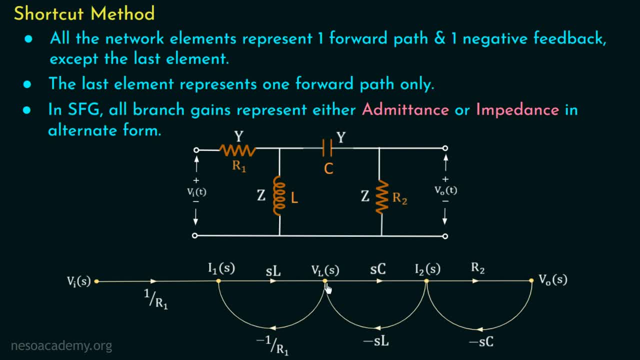 of this first element. Whenever we are connecting these two nodes, the branch gain will be the impedance of this second element. Then, when we connect these two nodes, the branch gain will be the admittance of this third element. And when we connect these two nodes, 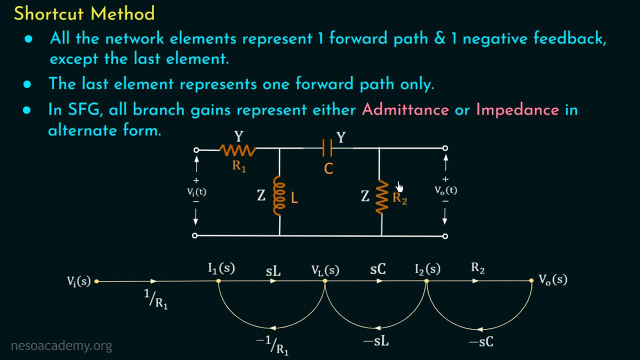 and the branch gain will be the impedance of this last element. In this way, we have completed our forward path. Now we have to remember one thing: that the last element represents one forward path only, So we have to use this element only one time, whenever we are creating the last branch of 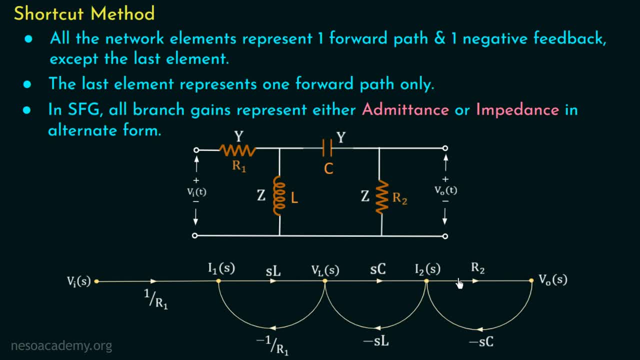 this forward path. Now, whenever we are connecting these two elements with a negative feedback, we will use this element and the branch gain of this negative feedback will be the admittance of this element, which is equal to sc. Similarly, when we will connect these two nodes with 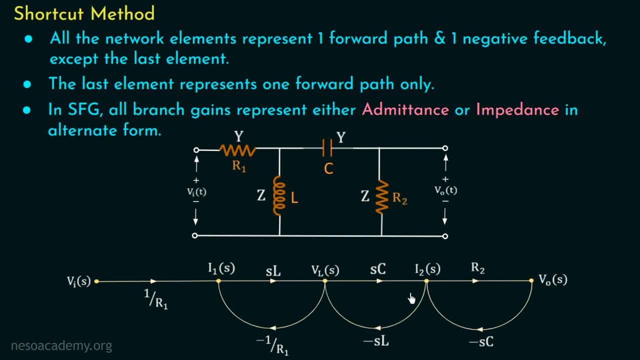 a negative feedback, the branch gain of this negative feedback will be the impedance of this element. And, lastly, whenever we connect these two nodes with a negative feedback, the branch gain will be the admittance of this element. I hope you got this Whenever. 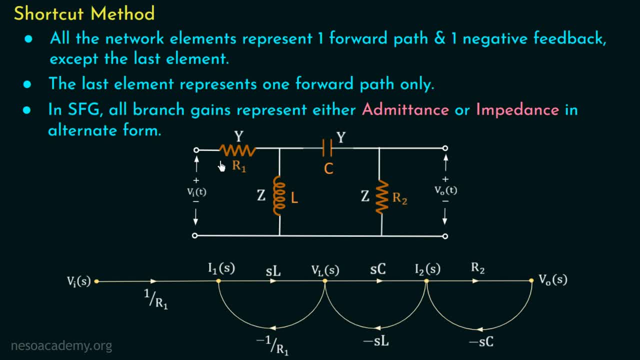 we are creating the forward path, we have to go in this order from left to right: admittance, impedance, admittance, impedance And then after that, whenever we are creating the negative feedback paths, we have to go in this order from right to left, except this element. So 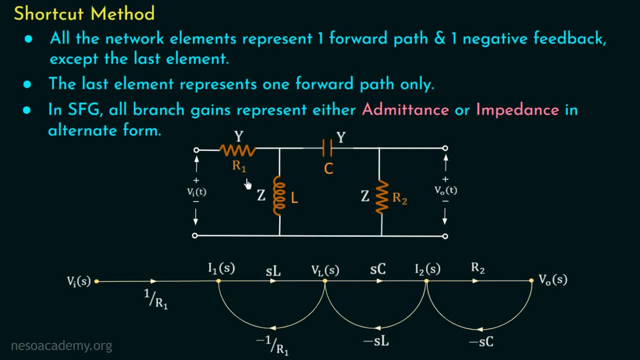 we will consider the admittance of this element, then the impedance and then the admittance. So in this way we have 4 elements. whenever we are creating the forward paths from the left to right, and hence we have 4 branches, But whenever we are moving back to create, 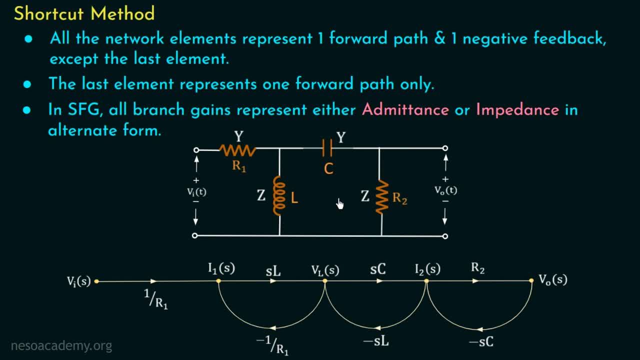 the feedback paths, we have only 3.. Since we do not have to consider this element and hence we have 3 different negative feedbacks, I hope you got this shortcut method. This is a very simple method by which we can draw the signal flow graph of any electrical network directly, If you solve some more problems. 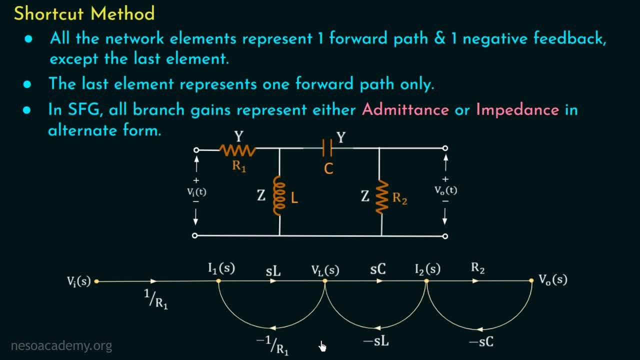 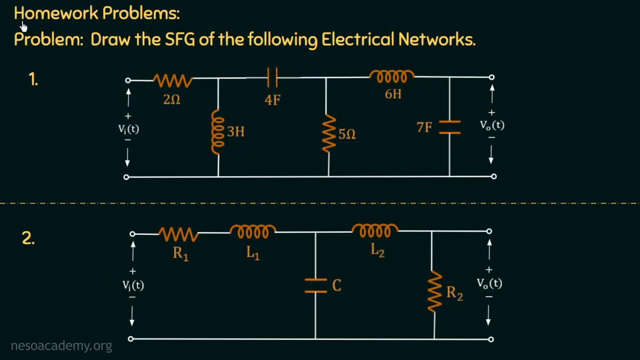 based on this method. you will find this method very simple And for that sake, I will give you some homework problems. So now I want you all to go through this method one more time And I will give you some homework problems based on this method.